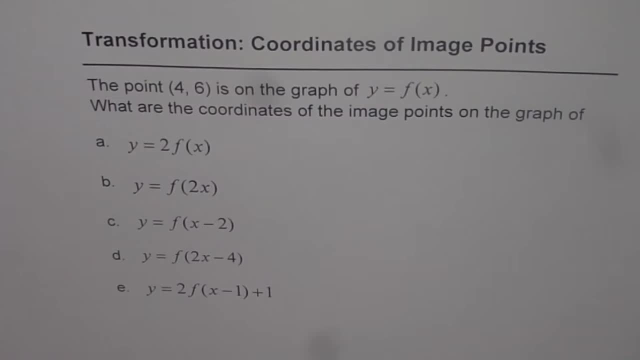 Here is a question to understand coordinates of image points on a transformed function. The point 4,6 is on the graph of y equals to f of x. What are the coordinates of the image points on the graph of? we are given five transformed functions, right So you? 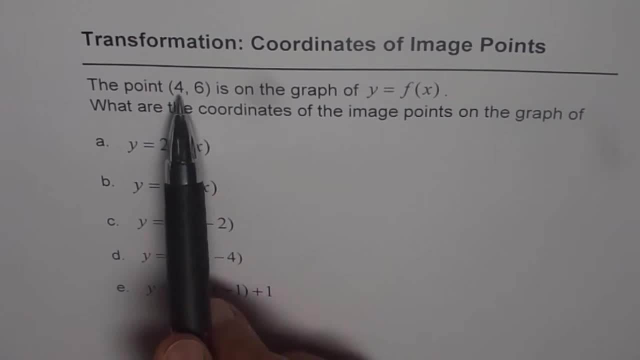 have to figure out on each graph how will this point 4,6 get transformed. So the first one is: y equals to 2 times f of x. Second is: y equals to f of 2x, And then y equals to f of x minus 2.. And then we have f of 2x minus 4.. And y equals to 2 times f of x minus. 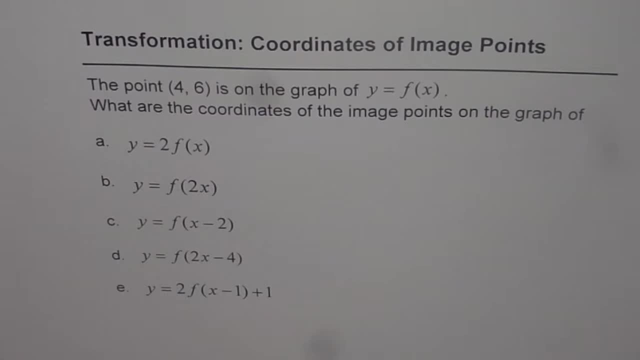 1 plus 1.. I'd like you to pause the video, answer the question and then look into my solution. So in the very first one, y equals to 2 times f of x. There is transformation, which is vertical stretch, by a factor of 2.. Now vertical stretch. 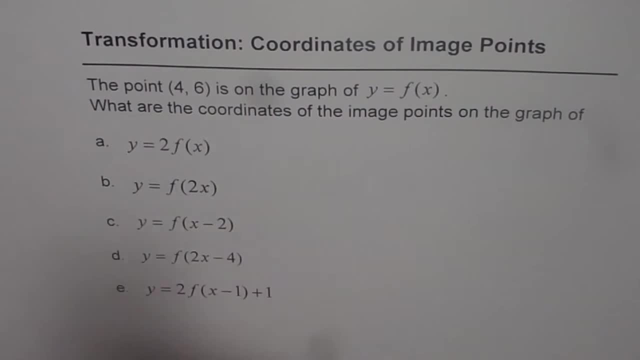 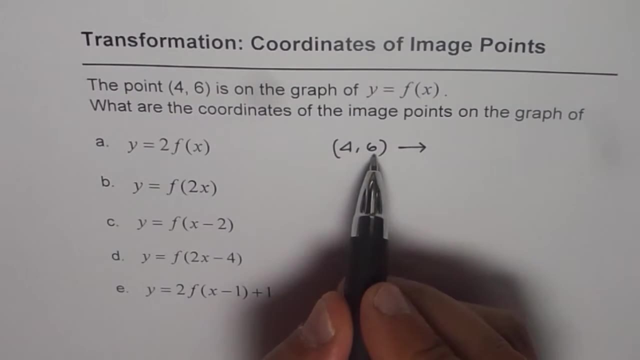 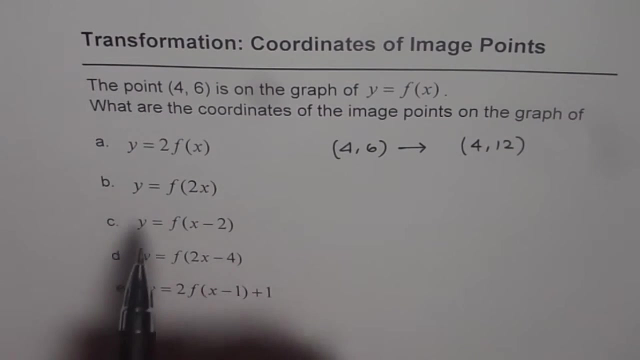 will only affect the y coordinate, correct. So the transformation is from 4,6 to the y coordinate gets multiplied by 2, so it'd be 4,12.. So that is a transformation. In the second case we have y equals to f of 2x. Here the transformation is horizontally. 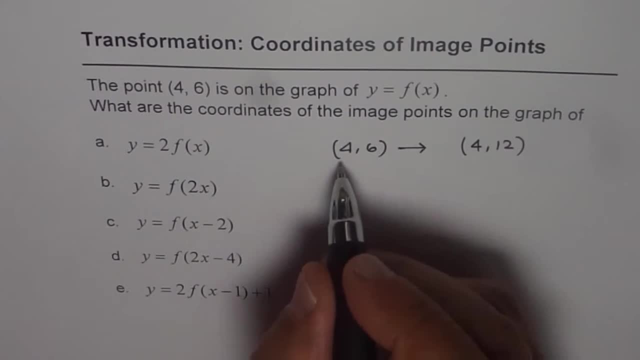 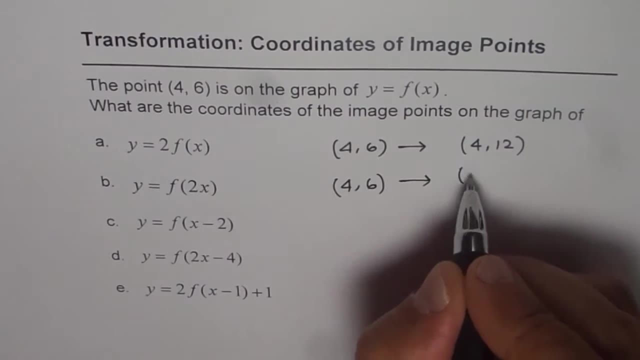 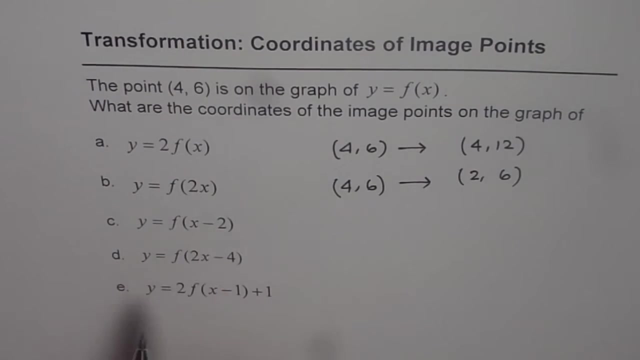 compressed by a factor of half, So the x point becomes half of the original value. Y point remains same, So half of 4 is 2, so we get 2 and 6.. C is y equals to f of x minus 2.. 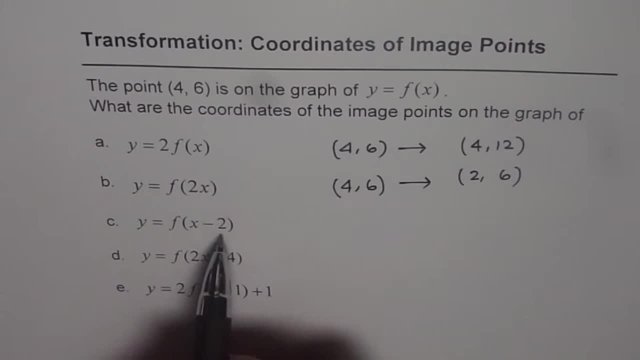 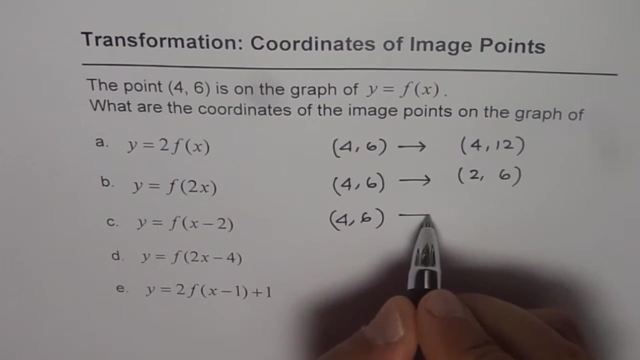 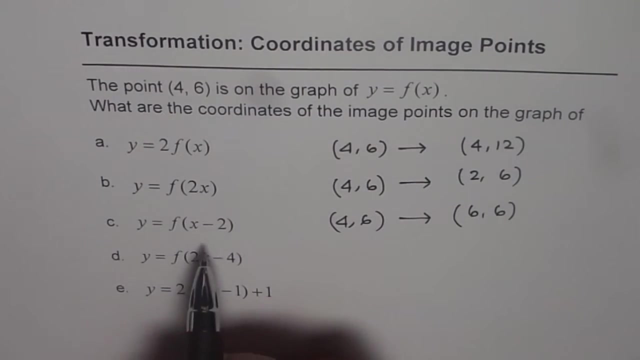 X minus 2 means a transformation which results in horizontal translation of two units to right, So the x points will get increased by 2.. Y remains same, So the original point 4,6 will get transformed, So 4 plus 2 will give me 6.. 6 comma 6 is the image point on the graph of the function. y equals to f. 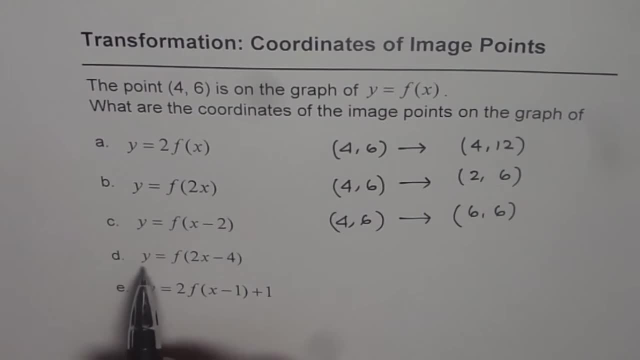 of x minus 2.. Now the next one is: y equals to f of 2x minus 4.. Now can you tell me how will this point 4, comma 6 get transformed in this particular case? Now, here it's kind of important to rewrite this in the factored form, which is f of let's. 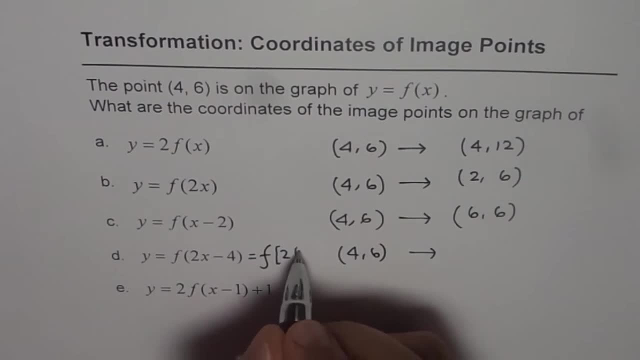 factor out 2.. If you factor out 2, you get x minus 2, right, So that is how you should do. Now it is horizontally compressed by a factor of half and then translated two units to the right. So what we do here is first we divide 4 by 2.. You can see that y equals to f of x minus. 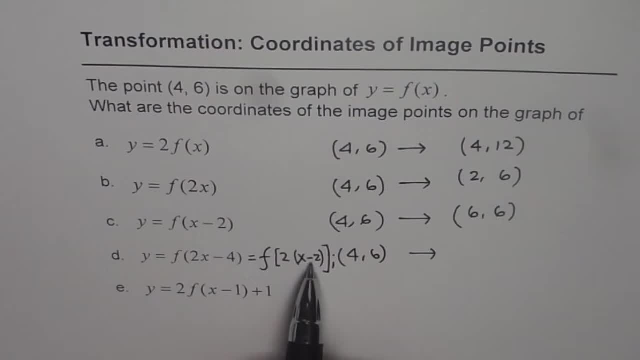 If you divide 4 by 2,, you get 2, and then you add 2, so you get 4 back. right, So 4, 6.. So this is the transformation which takes place. So first is dividing horizontally, compressed by a factor of half. 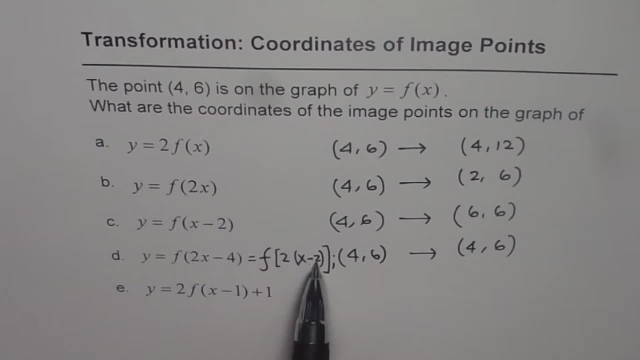 So half of 4 is 2, and then you add 2,, right? So when you add 2 to 2, it becomes 4.. So this point is invariant. It just is the same point, right. 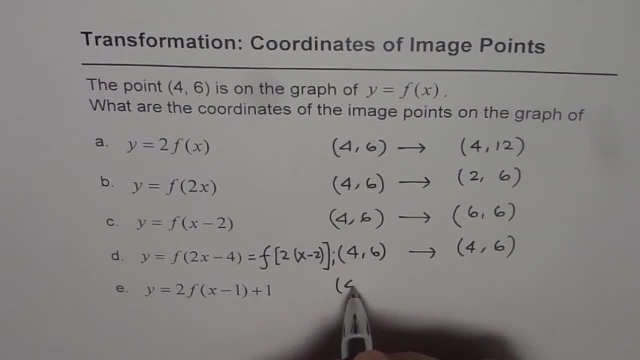 Now, in the next one here, what happens? The original point is 4,, 6, and the transformation is that the y values get multiplied by 2, and then you add 1.. For the x values you have to add 1, right. 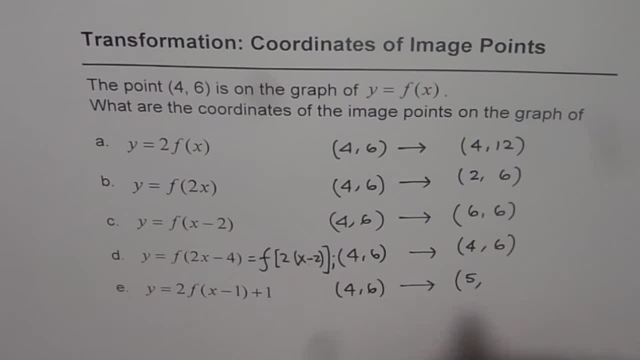 Minus 1.. So add 1 to 4 gives me 5, and for the y value we have to multiply by 2, and then plus 1.. Times 2 is 12, plus 1 is 13.. 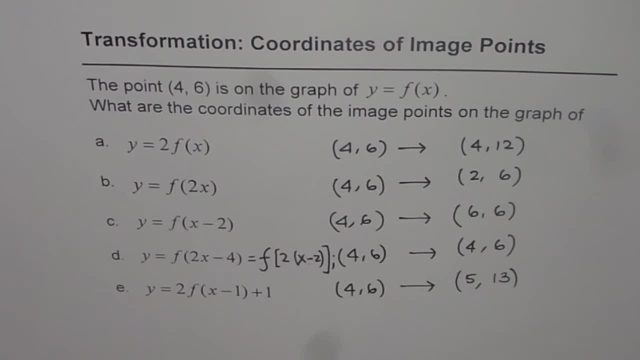 So it becomes 5, 13.. Right, So as an exercise, let me give you one question, and that is: y equals 2.. Let me just change this to half this time. and f of 2x plus, let's say plus 1, minus 1.. 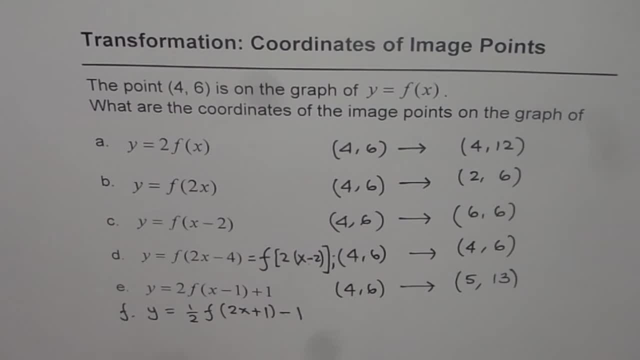 Okay, So write down the transformation of the coordinate point given to you- 4,, 6, on this function on the graph of this function. So that is an exercise for you. Okay, Thank you, Thank you.